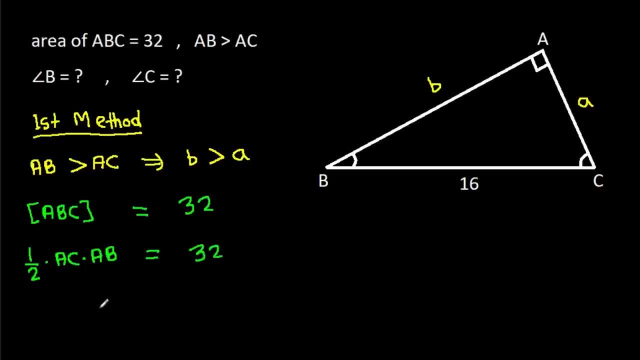 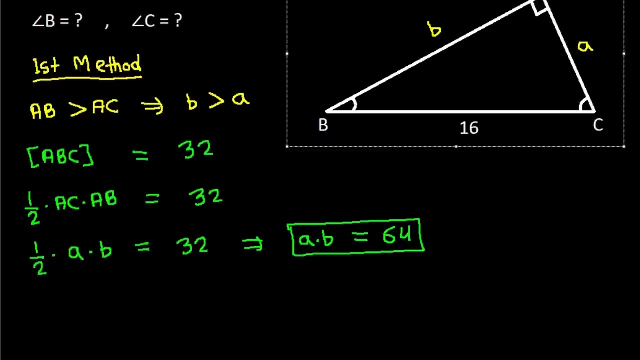 That is 32.. And it is 1 over 2 times AC is A Times AB is B, It is 32.. So A times B, It will be 32 times 2.. That will be 64. And 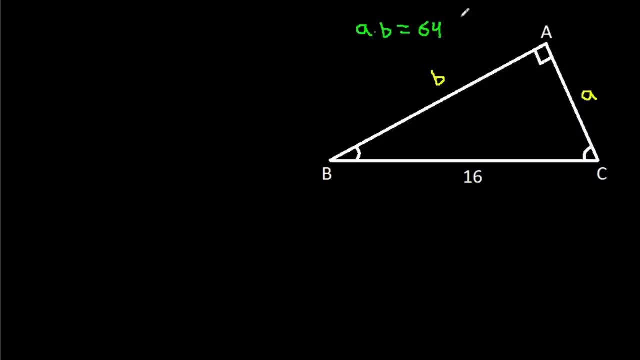 We get A times B is 64.. And AC square plus AB square, It will be equal to BC square by Pythagoras theorem. And AC is A square plus AB is B square. It is equal to And BC is 16 square. 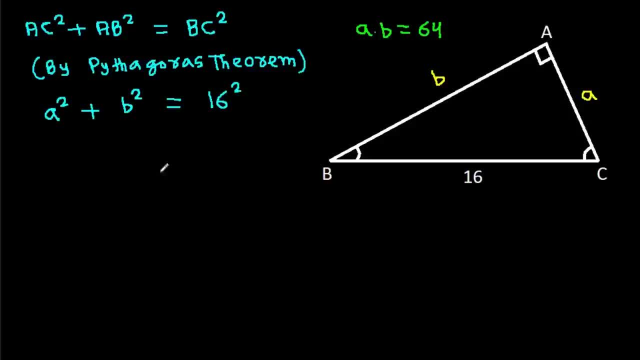 And we know that A plus B square It is equal to A square plus B square plus 2 AB. And A plus B square It is equal to, And A square plus B square, It is 16 square plus 2 times. 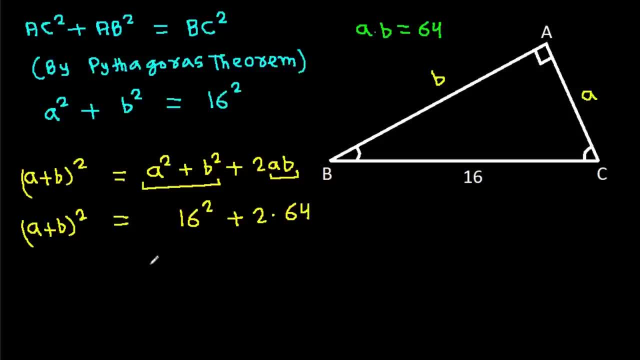 And AB is 64.. And A plus B square It is equal to: And we can take 16 common And it will be 16 plus 2 times 4.. And A plus B square, It is equal to 16 times. 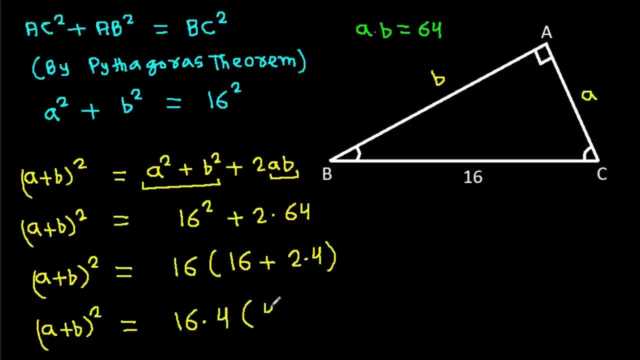 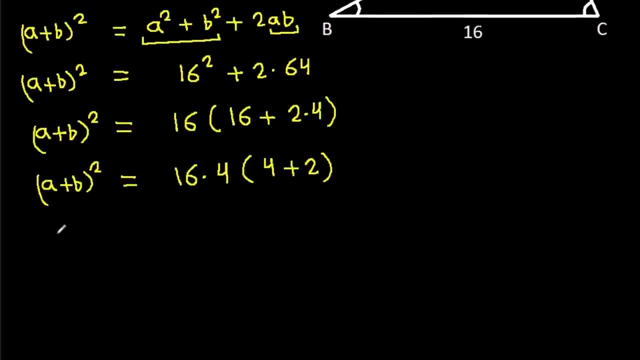 And we can take 4 common And it will be 4 plus 2.. And And A plus B, A square It is 64 times 6.. So A plus B, It will be root under 64 times 6.. 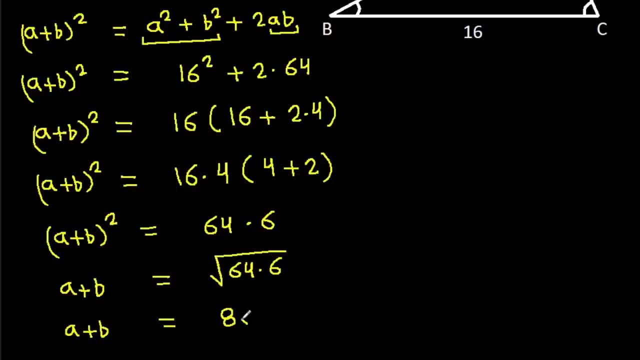 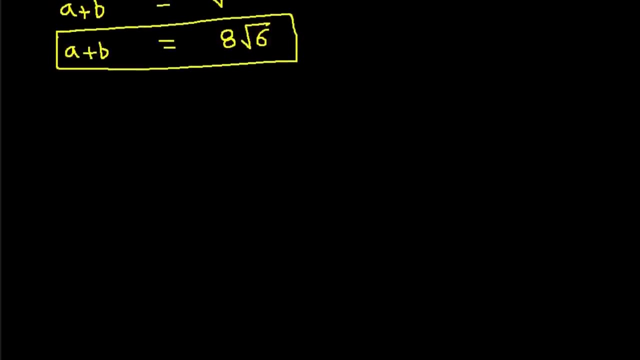 So A plus B, It will be at root 6.. And And and we have a b is 64, we have a plus b is 8, root 6 and a, b is 64. and for equation x square minus alpha plus beta, x plus alpha beta is equal to 0, the root. 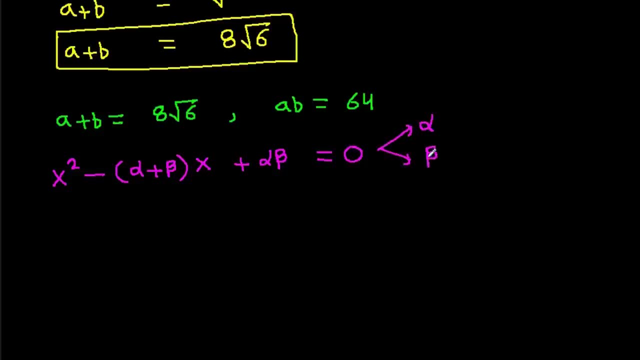 of this equation is alpha and beta. so for equation x square minus a plus b, x plus a, b is equal to 0. the root of this equation will be a and B and it is x square minus a plus b is at root 6. x. 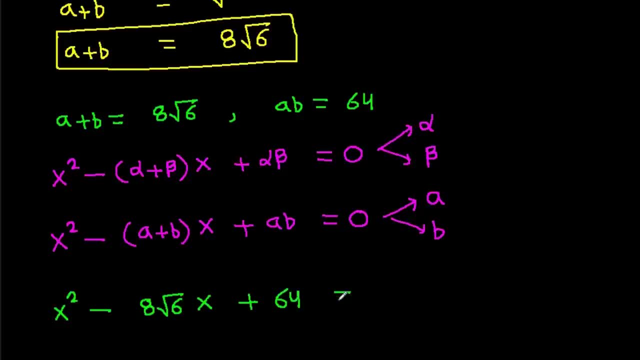 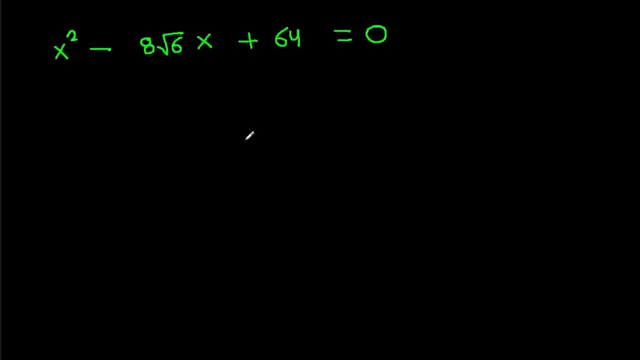 plus a, b is 64, it is equal to zero. and now for equation: AX square우 plus bx plus c is equal to 0.. x is equal to minus b plus minus root under b square minus 4ac over 2a, And here a is 1, b is minus 8 root, 6 and c is 64.. So x it will be minus. 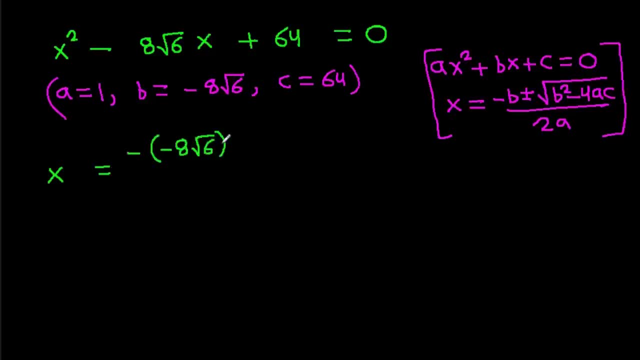 times minus 8 root, 6 plus minus root under, b minus 8 root, 6, square minus 4 times 1 times 64 over 2 times 1.. And x is equal to 8 root 6 plus minus root under, and this will be 64 times 6 minus. 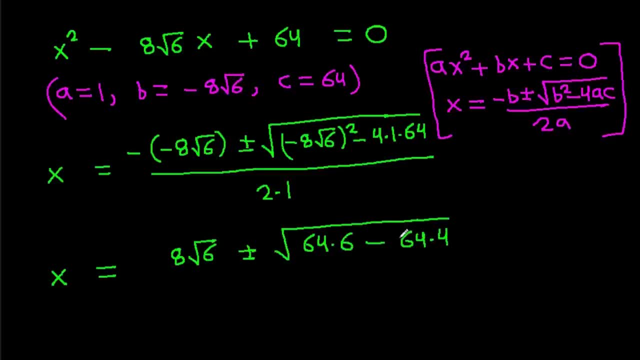 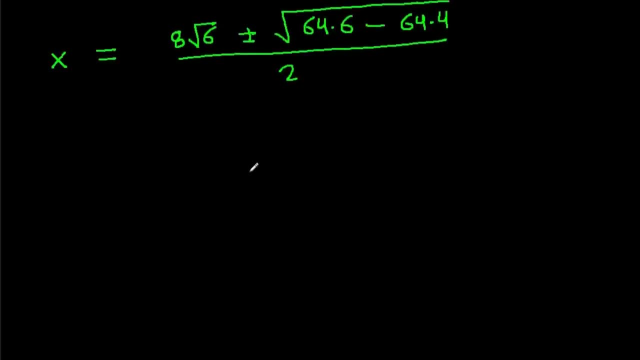 64 times 3 over 4.. It will be 64 times 2 over 64, minus 64 times 3, and 64 will be 64 times 3 over 4.. It will be minus 64 times 4 over 2 over 6in. It will be powerful. k is equal. 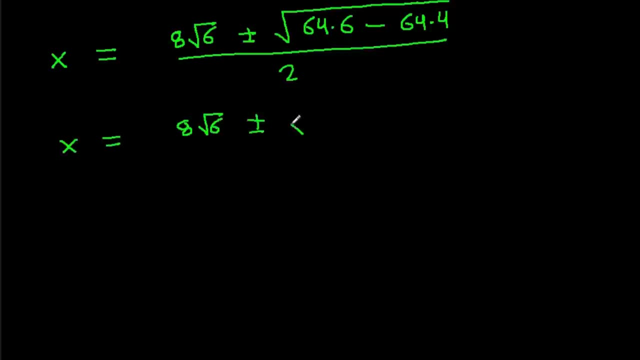 to minus 6metallic time. slash the square minus c, So here a is 16 plus 54 times 3, power minus 64 times 4. And there will be over 2 minus 64 times 4 over 4.. And here x is equal to 8 root, 6 plus minus root under b And 64. 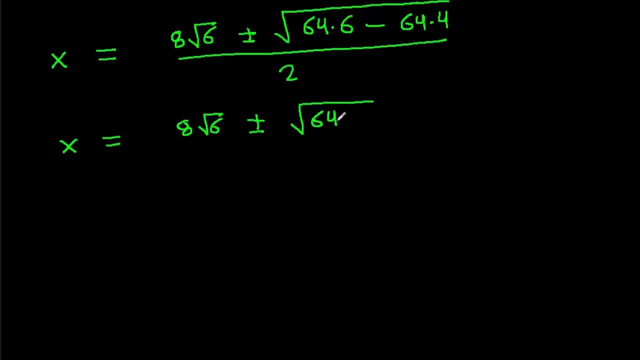 times 4 over by from 64 times 64 minus 64 times 4.. It will be 64 times 2 over 64 plus minus 64 times 4 over 2.. Nil, my time remember We have been doing several jederaders with. 44. i saw you doing send manhandshat because we didn't know well how to do verb contempt. number 8: root x minus 64 plus minus minus, this is 64 times 4 over b. And the last solution in this: 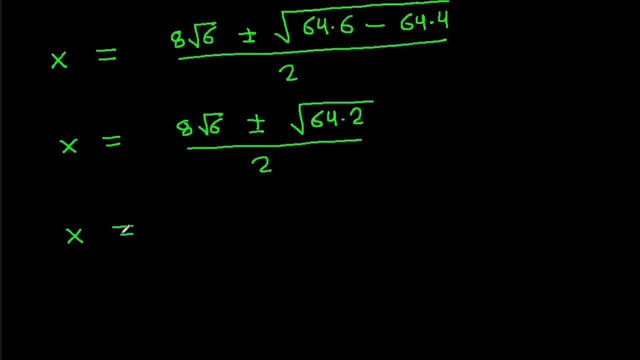 over 2 and x is equal to 8 root 6 minus minus 8 root 2 over 2. and if we divide by 2 then x will be equal to 4 root 6 minus minus 4 root 2 and x is equal to. we can take 4 root 2 common and it will be root 3 plus minus 1. 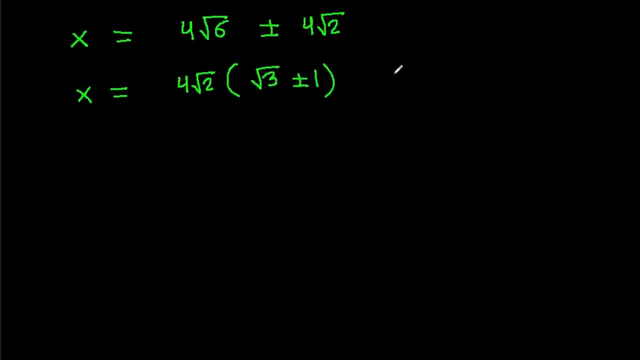 and we know that the root of the equation was a and b. so from here, either a it can be 4 root 2, or it can be root 3 plus minus 1. and we know that the root of the equation was a and b. so from: 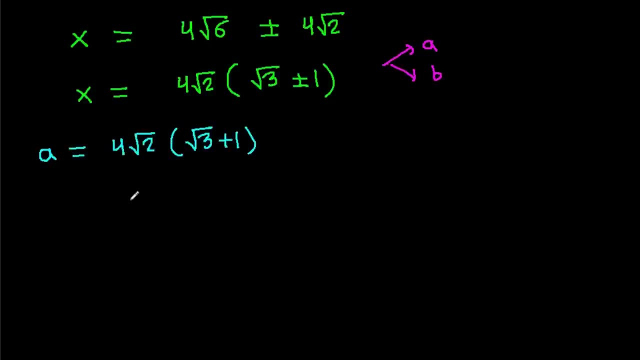 2 times root 3 plus 1, and b- it can be 4 root 2 times root 3 minus 1, and either: a- it can be 4 root 2 times root 3 minus 1, and b- it can be 4 root 2 times root 3 minus 1. 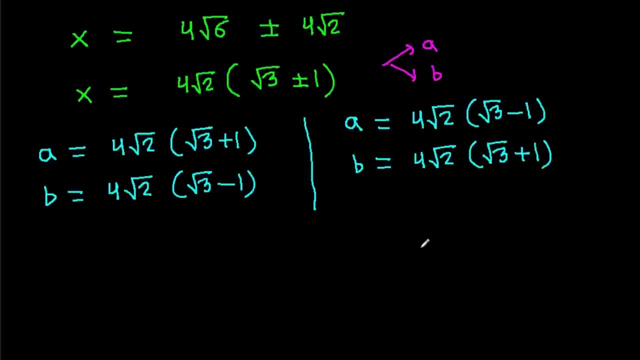 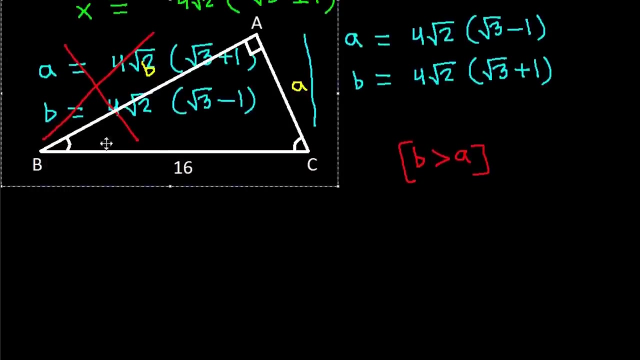 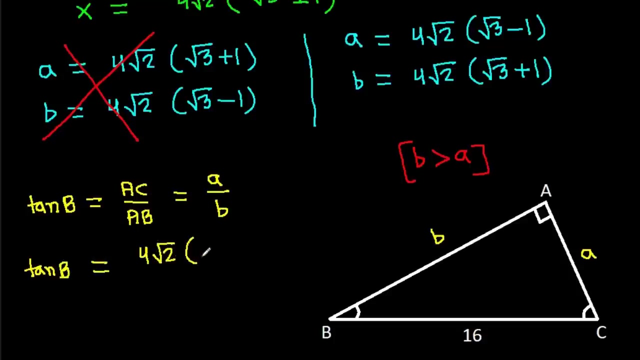 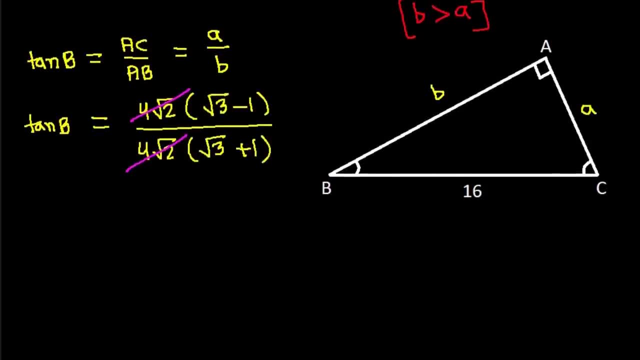 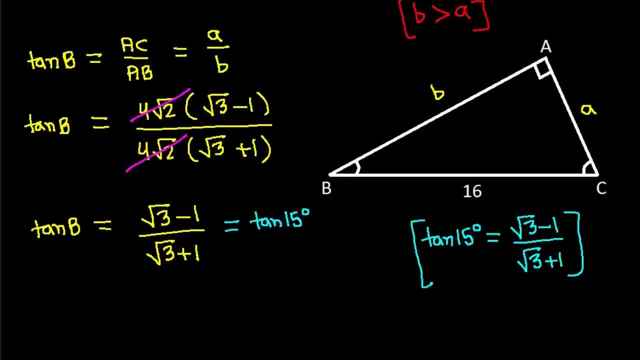 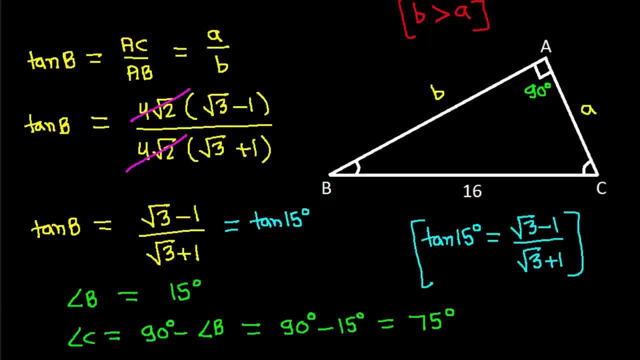 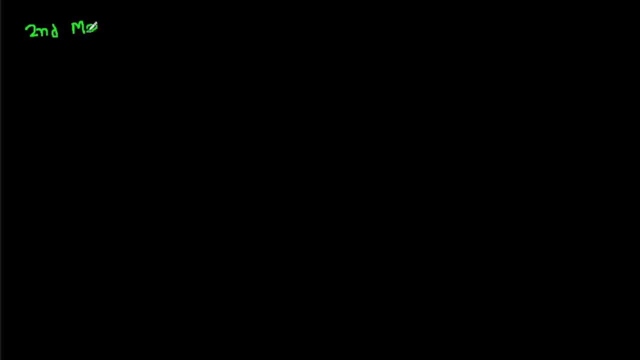 so it will be 75 degree. and the second method we have: area of abc is 32 and bc is 16, and suppose d is midpoint of bc, then bd- it will be equal to cd. bd: it is equal to cd, it is our construction- then bd- it will be equal to cd. 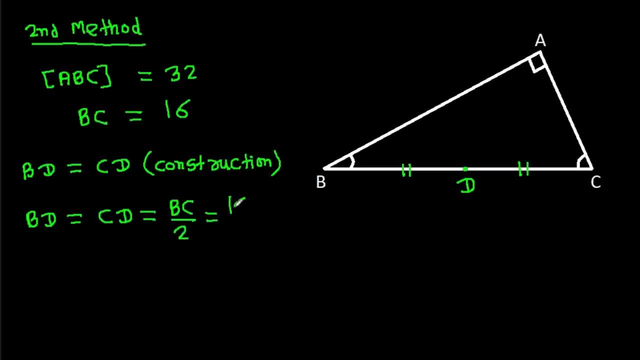 that will be bc over 2 and bc 16 over 2, that will be 8. so bd is 8 and cd is 8 and if we join ad then In any circle diameter diameter makes an angle of 90 degree on the circle and here 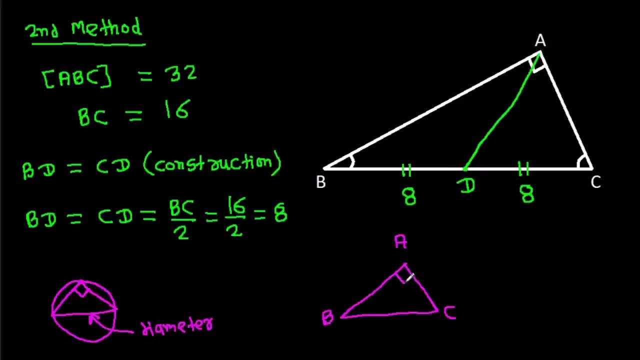 inter angle ABC. this angle is 90 degree and if we make a circle around ABC then we know that angle BSC is 90 degree. that means BC, it will be diameter, and D is midpoint of BC, and then BD, it will be equal to CD and will be equal to AD. that will be radius. 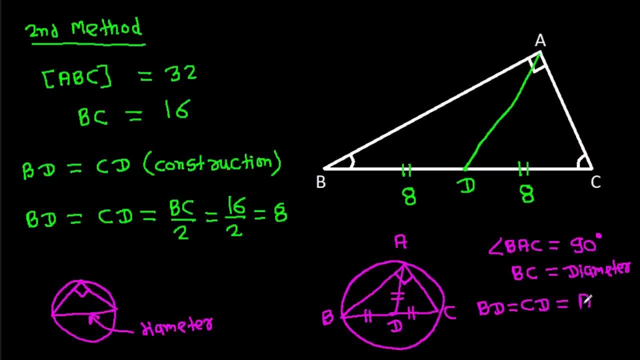 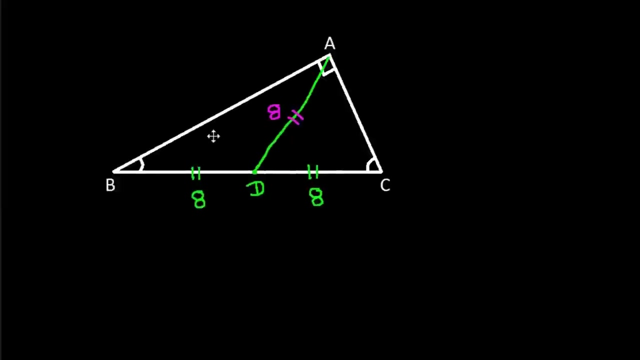 BD, it will be equal to CD, it will be equal to AD. that will be radius, so AD it will be also 8. and Now inter angle: ABD it is ABD we have. BD is equal to AD. That means these two angles, they will be equal. 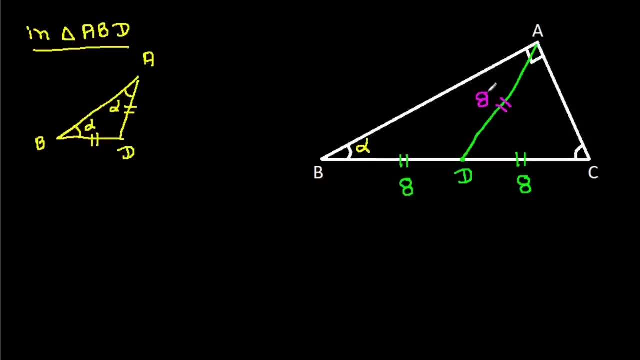 Suppose ANPHA, if this angle is ANPHA, then this angle it will be also ANPHA. And from point A, if we make a perpendicular on BC, suppose this point is E and we have CD is 8. And we know that area of ABC is 32.. 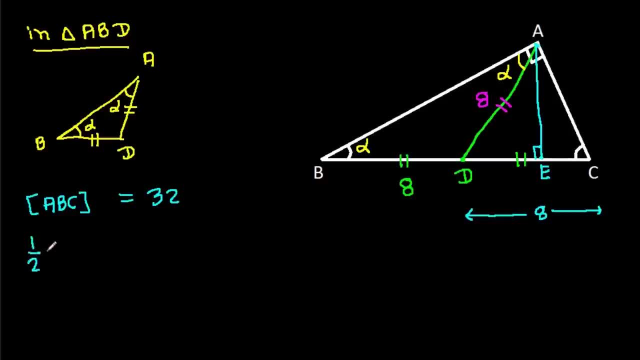 And area of ABC. it will be 1 over 2 times base is BC and height is AE. that is 32.. And it is 1 over 2 times BC is 32.. That is 32.. So from point A it will be 2 over 2 times BC is 16 times AE, it is 32.. 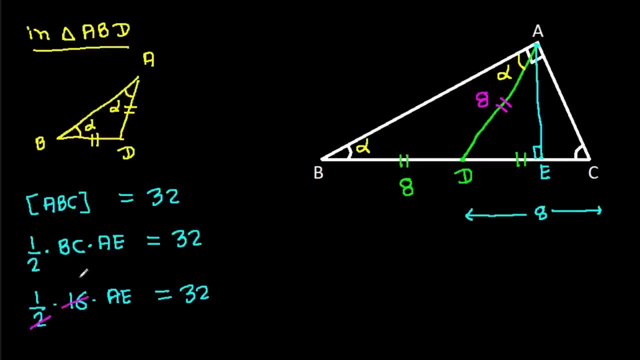 And 2 times 8 is 16, and 8 times 4 is 32.. So AE it will be 4.. AE is 4.. And 8 times 4 is 72. So AE it will be 4.. 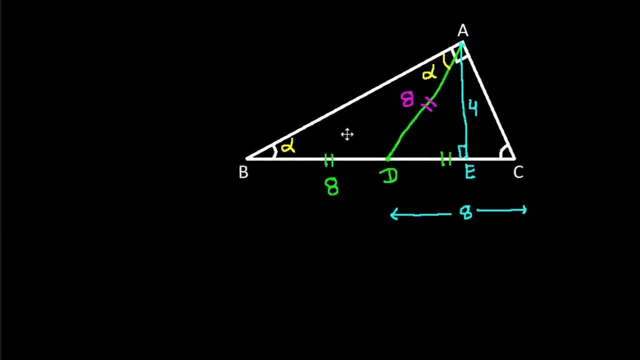 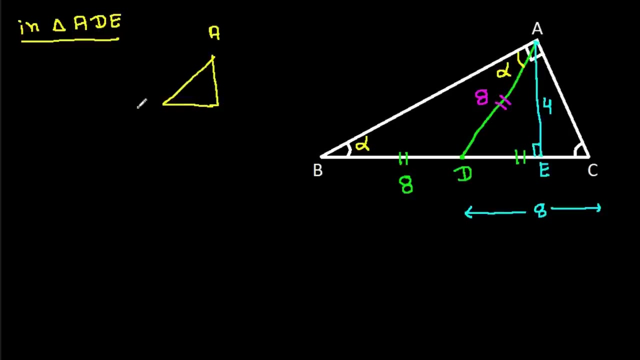 Now inter angle: ADE: it is ADE, AE is 4, AD is 8 and this angle is 90 degree and ADE, and suppose this angle is theta, then, Sineθ, it will be AE over AD and AE is 4 over AD. 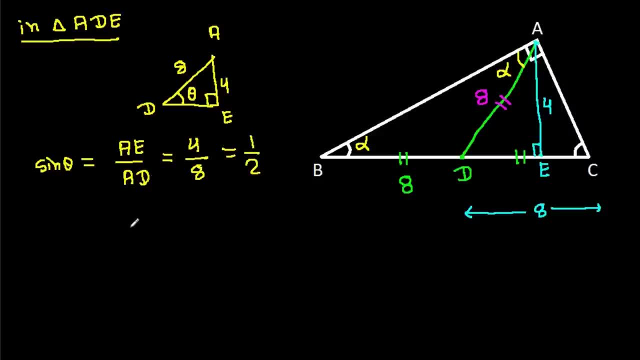 is 8 and it is 1 over 2, that means θ, it will be 30 degree. This angle, it will be 30 deg. And now inter angle, ABD, this angle is alpha, this angle is alpha and this exterior angle. 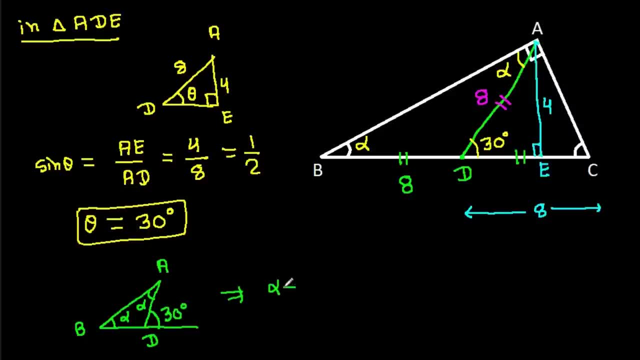 it is 30 degree. So alpha plus alpha it will be 30 degree, So alpha it will be 30 degree over 2, that will be 15 degree. this angle, it is 15 degree, and we have alpha is angle B, that is 15 degree, and angle C it will be 90 degree minus angle. 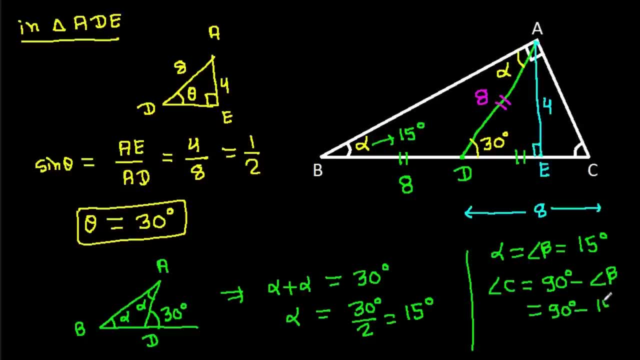 B, that will be 90 degree. So angle C, it will be 75 degree.